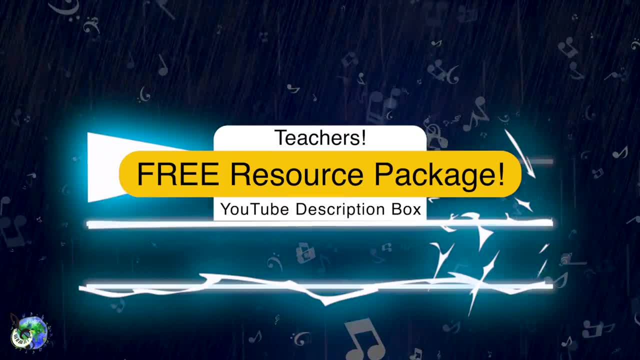 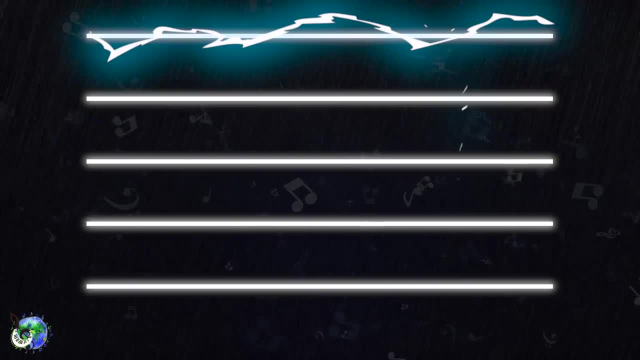 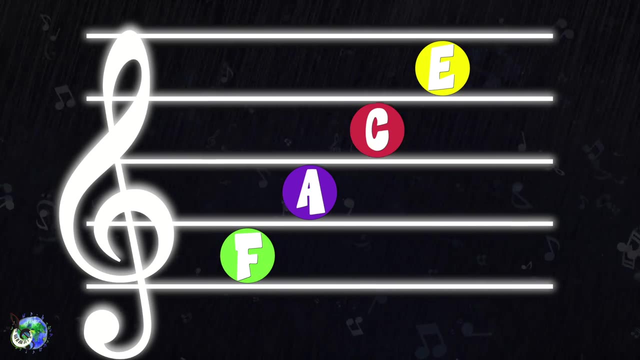 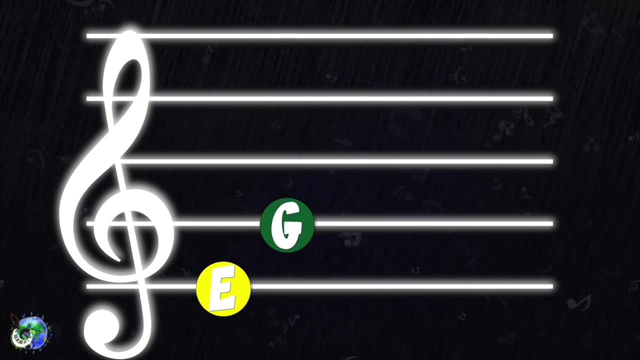 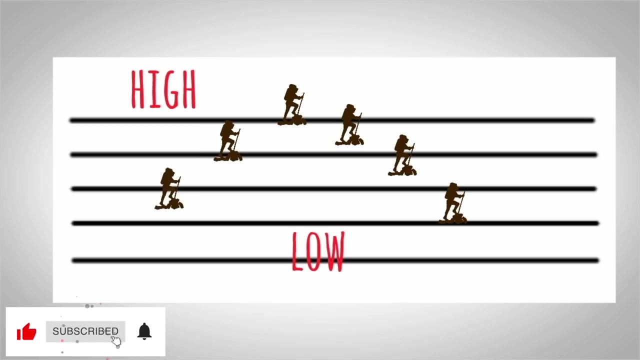 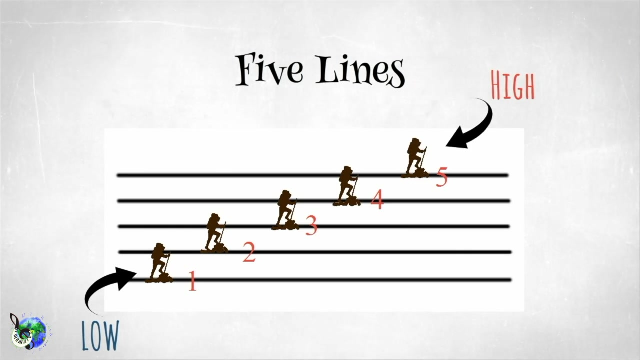 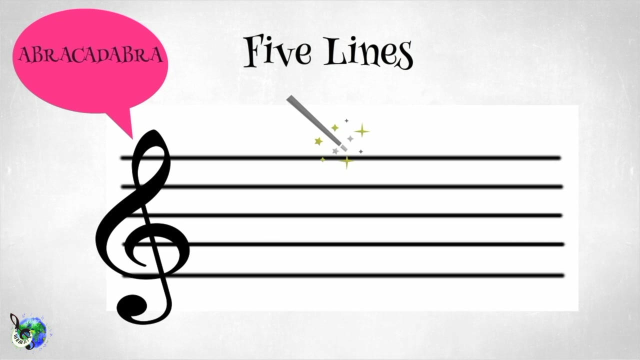 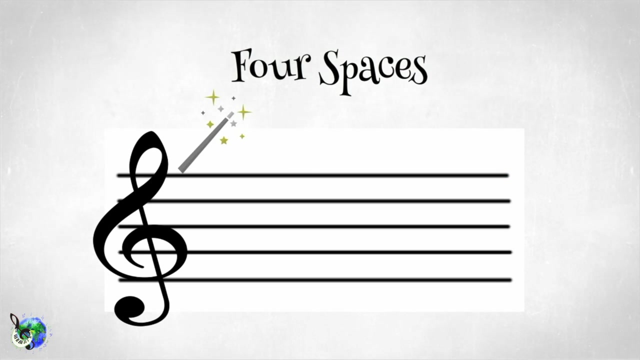 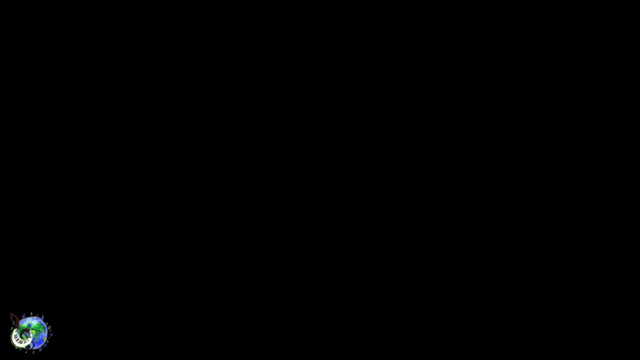 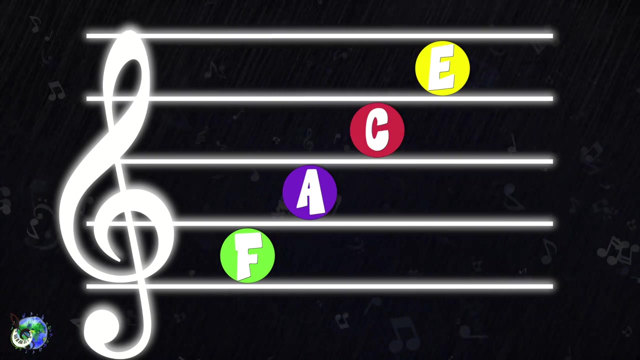 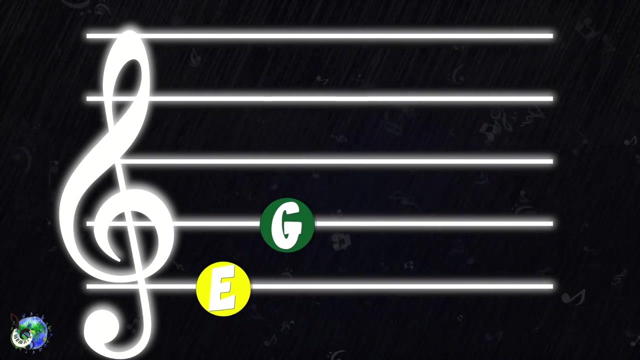 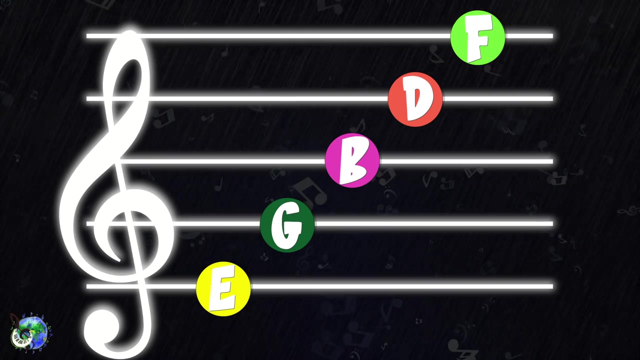 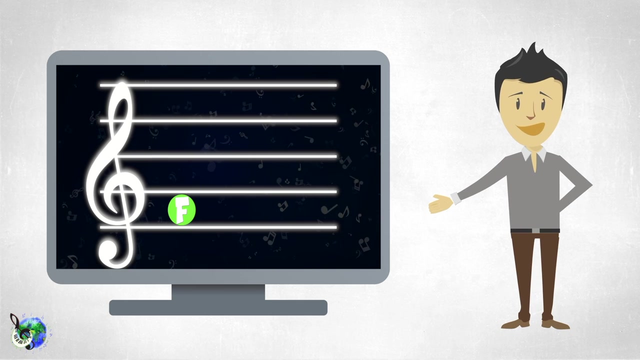 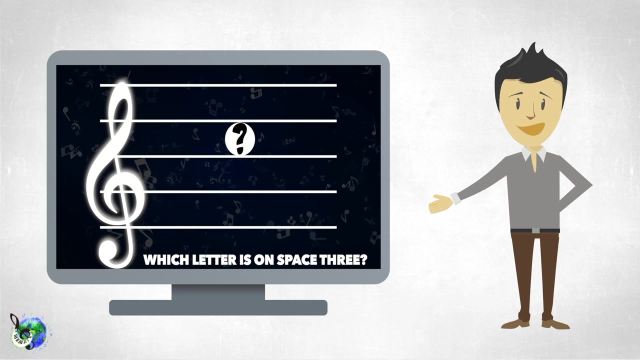 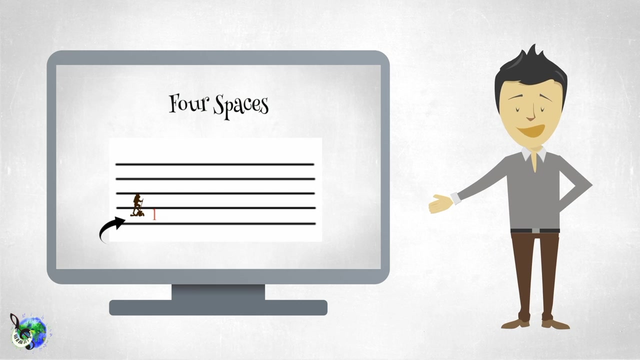 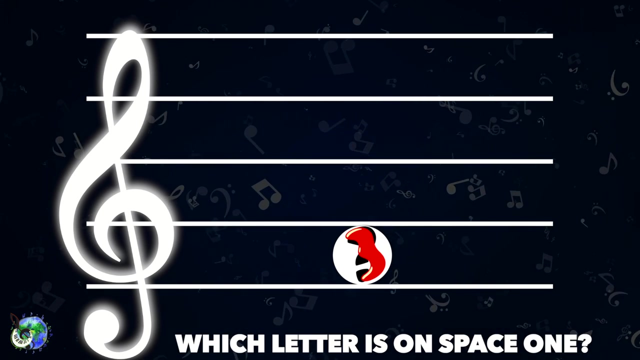 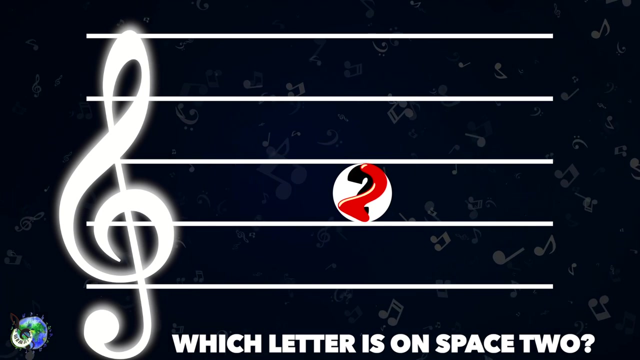 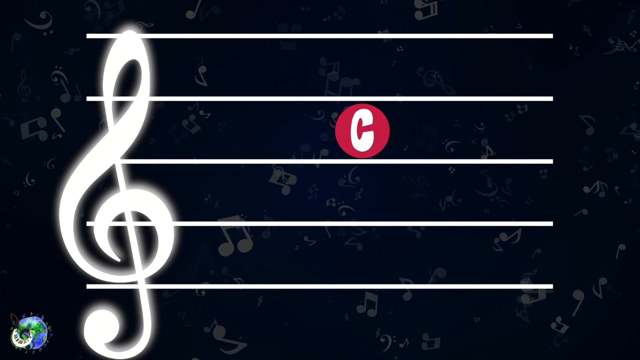 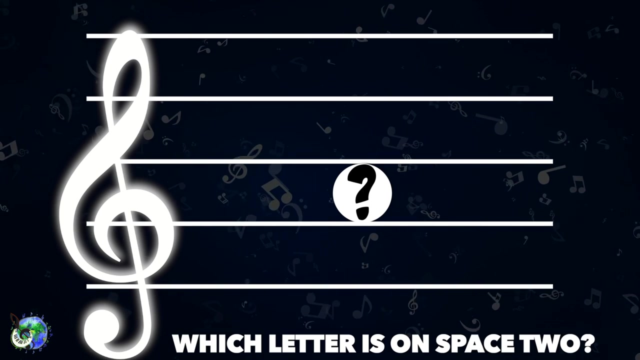 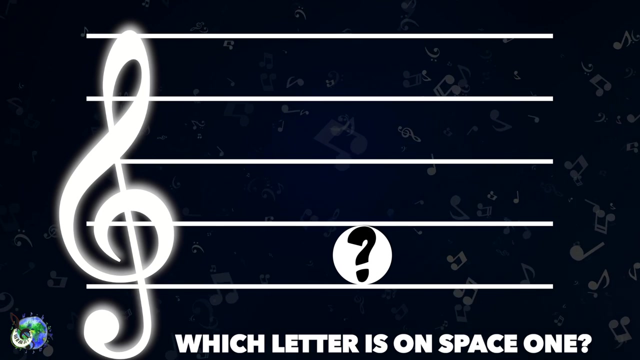 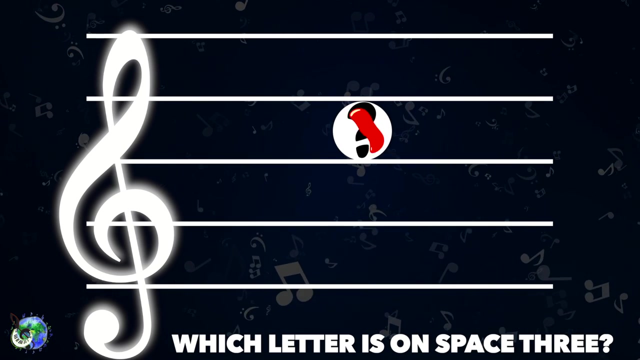 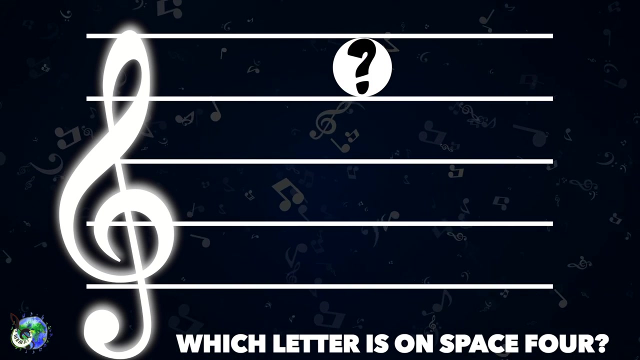 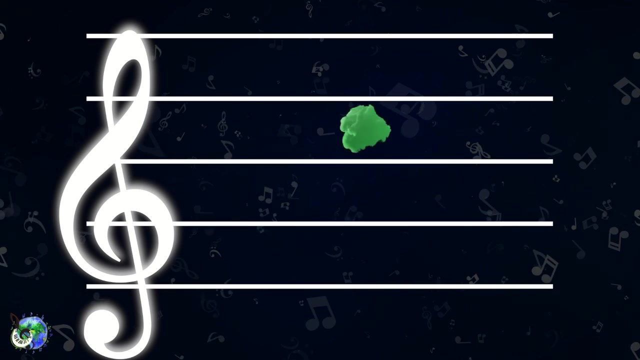 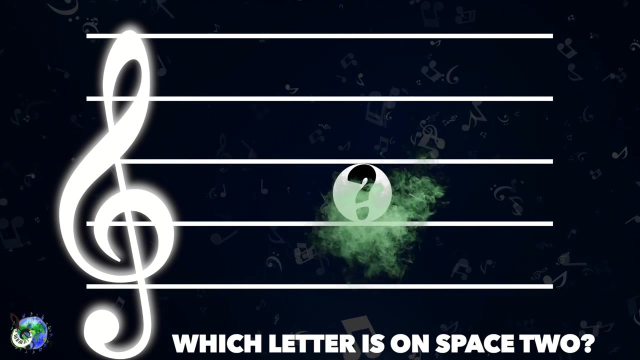 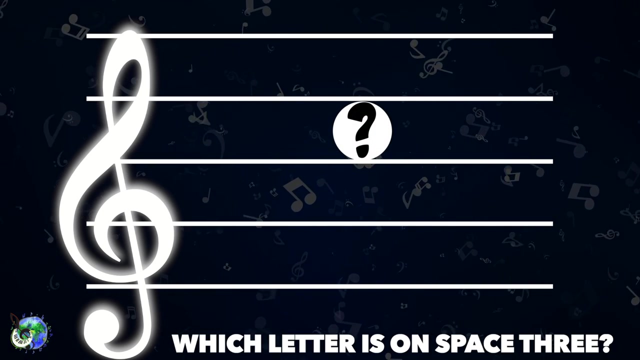 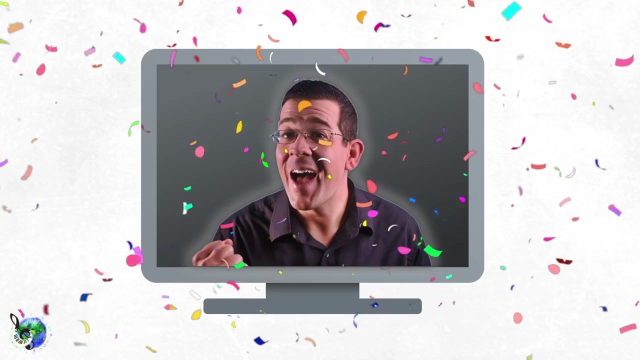 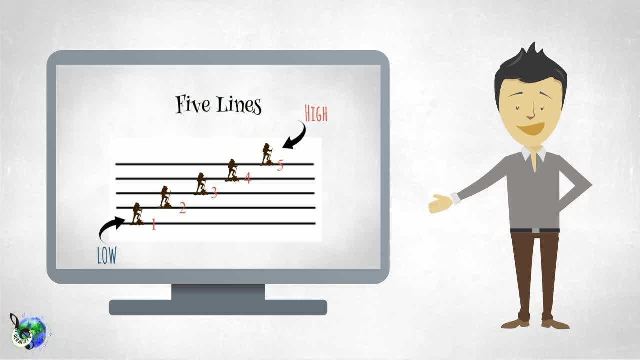 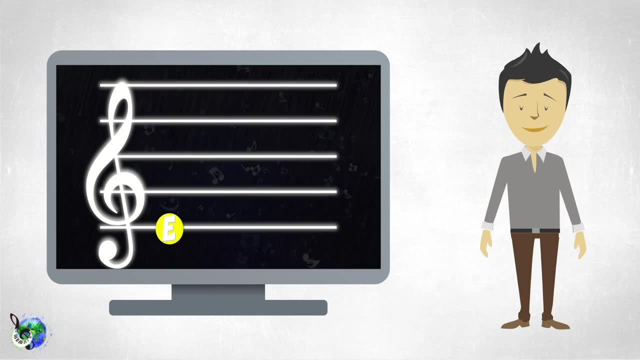 Remember. line one is at the bottom of the staff, then two, three, four and five. To help remember and figure out which letter is on the line, just think back to the rap with an E and a G and a B, D, F. 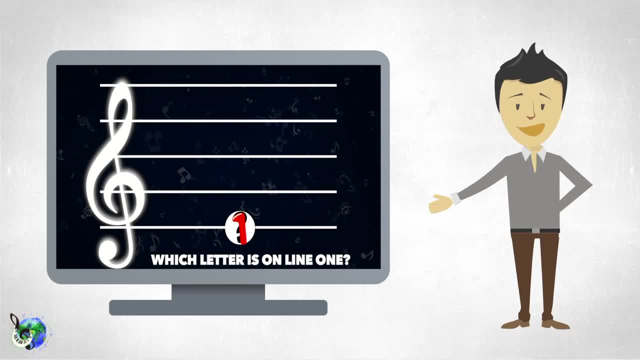 You will hear a line number called out and then a countdown of three. Your job is to say the correct letter out loud, right in time with the music. after the countdown of three: two, one. Here we go. Which letter is on line one? 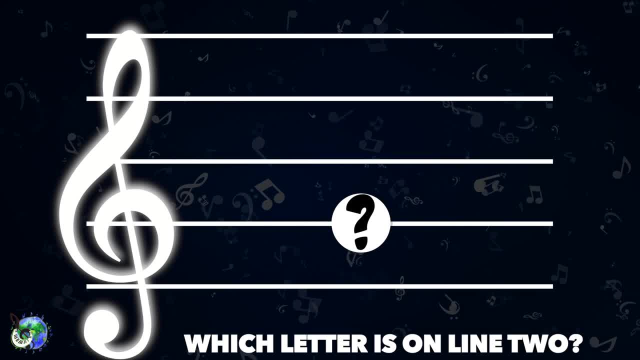 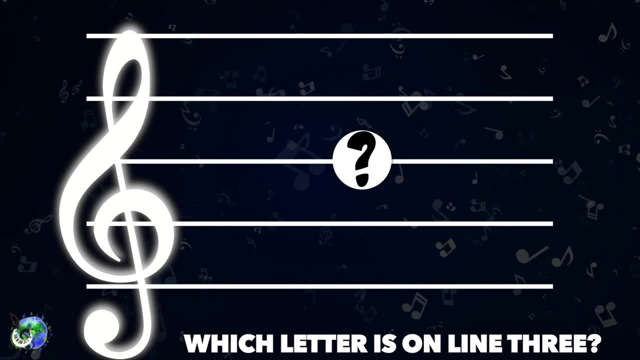 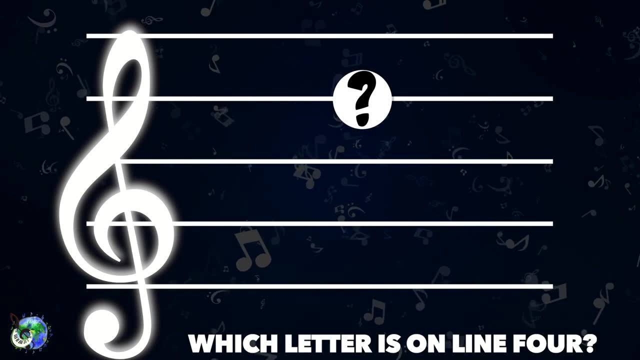 Three, two one E. Which letter is on line two: Three, two one G. Which letter is on line three: Three, two one B? Which letter is on line four: Three, two one D? 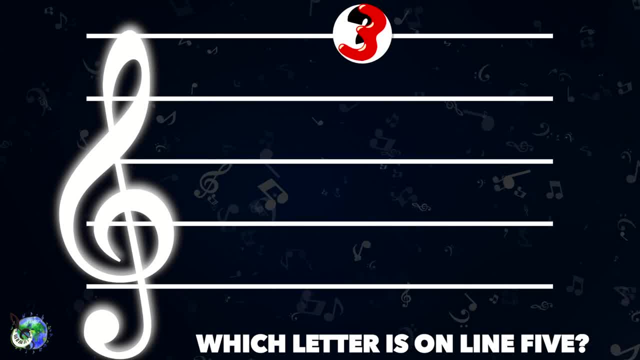 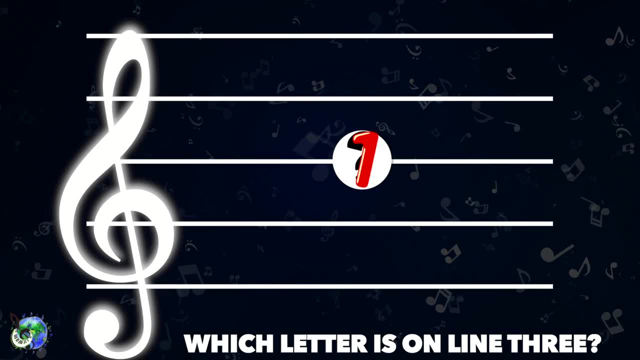 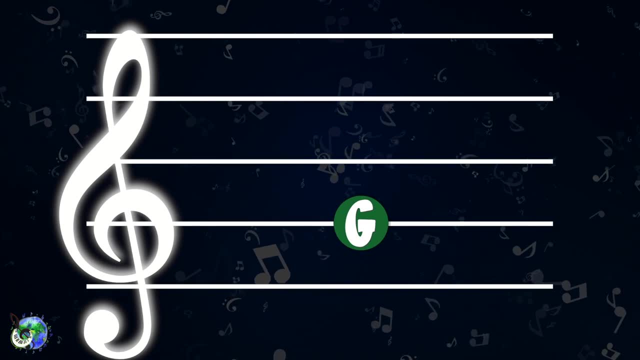 Which letter is on line five, Three, two, one F. Which letter is on line three, Three, two, one. Which letter is on line two, Three, two, one. Which letter is on line five, Three, two, one? 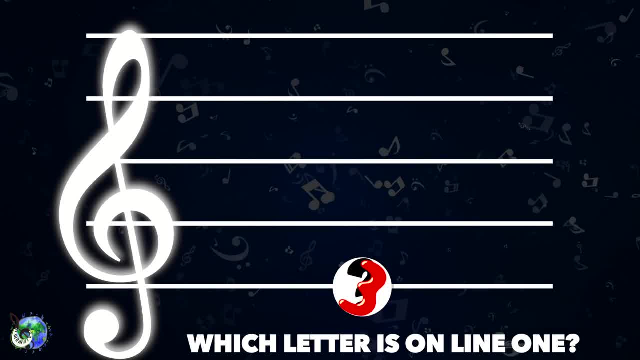 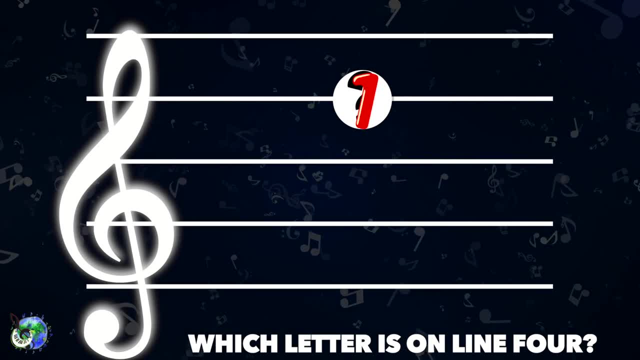 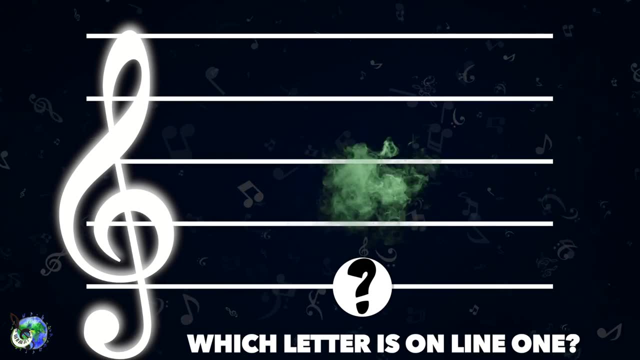 Which letter is on line one, Three, two, one. Which letter is on line four: Three, two, one. Which letter is on line two, Three, two, one. Which letter is on line one, Three, two, one? 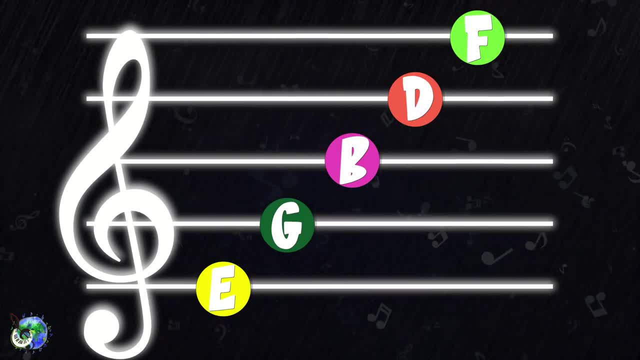 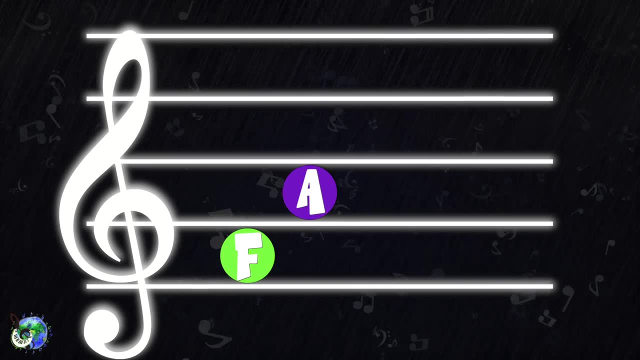 With an E and a G and a B D F, With an F and an A and a C E. With an E and a G and a B D F, With an F and an A and a C E. 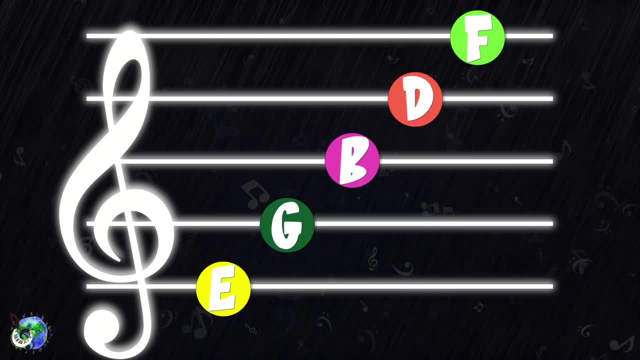 With an E and a G and a C E. With an E and a G and a B D F, With an F and an A and a C E, With an E and a G and a B D F. 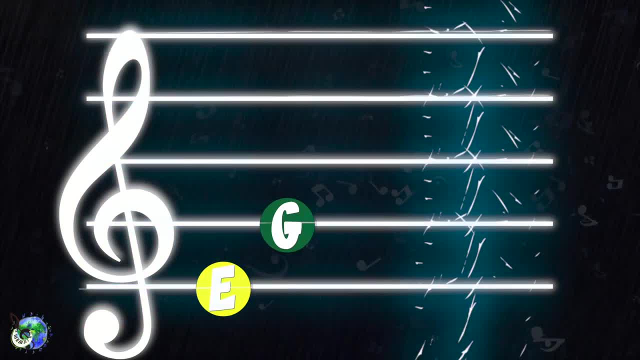 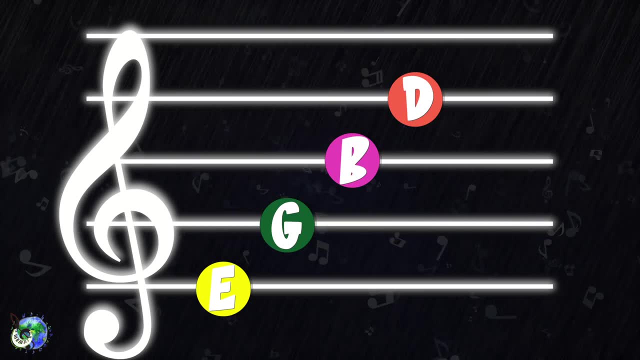 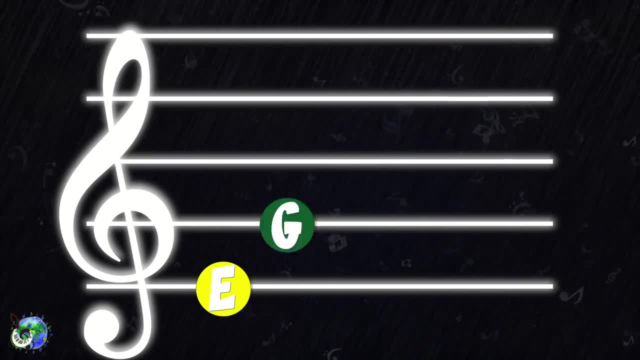